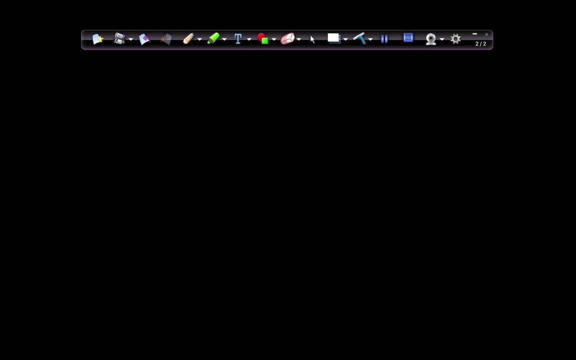 Welcome to my new video, and in this video we will be seeing what is TF-IDF and how it works, and what is the mathematical formulation of TF-IDF, and then we will see how to use the TF-IDF Vectorizer class provided by the ASCII. Learn to vectorize our data and why TF-IDF is better than Bag of Words. 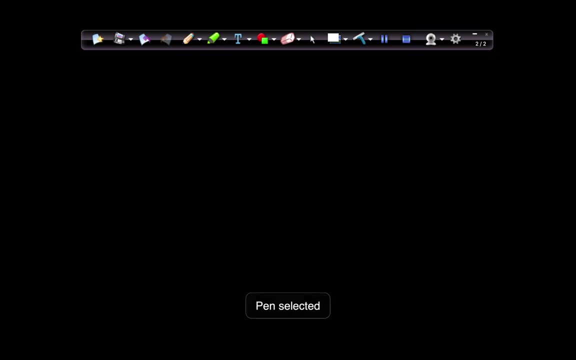 So lets start. So this particular term, TF, This is term frequency and idf is inverse document frequency. Now, what is term frequency? The term frequency for theoloidbook here is 1-3-4-1566. The term frequency in general is number of times. 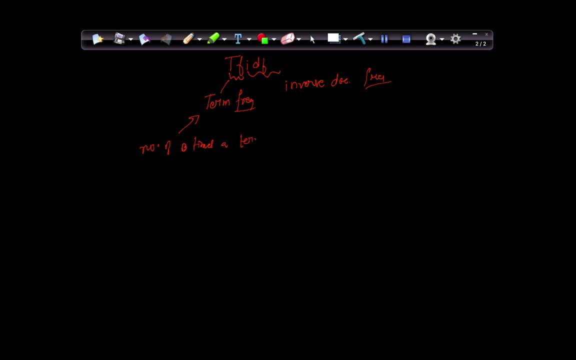 The term frequency in general is number of times, The number of times, Number places, The number places times, a term. what is term? term is word. word occurs in a occurs in a particular document, in a document. this is term frequency. what is inverse document frequency? inverse document frequency is log of n upon D. now, what is n? n is total. 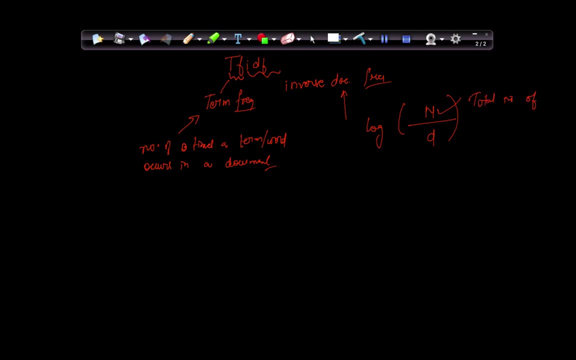 number of documents. this is total number of documents. and what is D these number of documents? number of documents in which term was present term or particular word for which we are calculating tf-idf is or was present. so now why we are taking this point: particular term. let me explain it okay, suppose, suppose we have d1 document, d2 document, d3 and 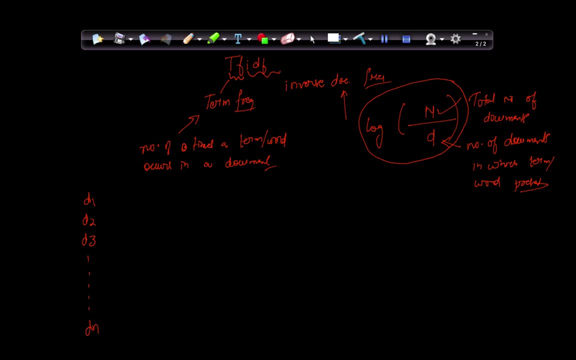 dn document and suppose there is a word w. this word occurs only in 10 or 20 of the documents, and suppose there are thousand documents. suppose there are thousand documents and a particular word occurs only in 10, 20 or suppose 50 documents, then this word, this word, this particular word may. 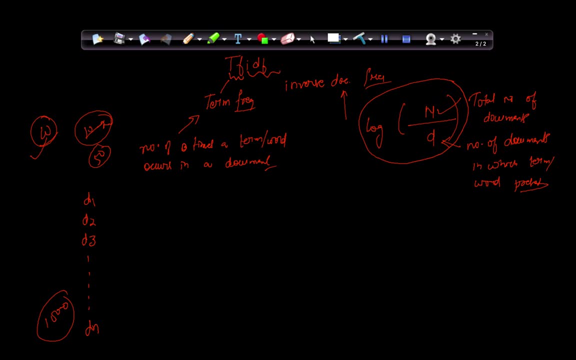 be very much informative, because rare words are informative, suppose, in the whole of the corpus. if some of the words are very there, then we have to give more weightage to them because they contains more informative, sorry, more information about that particular document. because if a document suppose is, if this d1 document or suppose this d2 document is different from these documents, 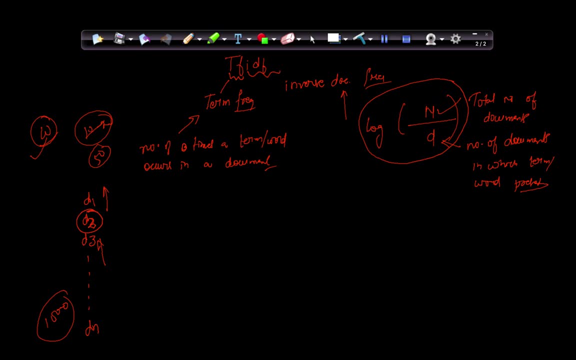 then how to decide this? so, in order to decide whether a document is different from others, there is only one way, and that is to gather information or to collect information from this particular d2 word. now suppose, suppose d2 contains 10 words, suppose d2 contains 10 words that are very rare in this particular corpus, then if, if the user query, if, 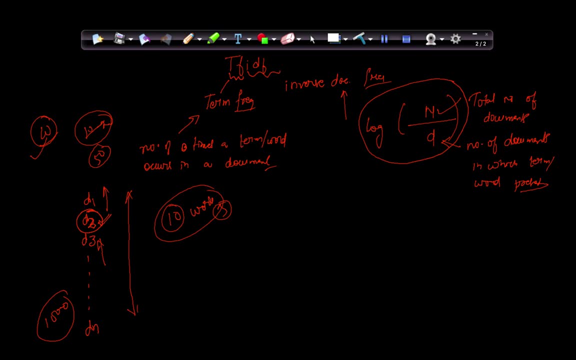 the query given by the users contain three words, three words among from this particular 10 words, then we will. we can directly say that, yeah, the user is searching from. the user is searching for this particular document. how? because the query of the user contains three words that are very rare in this whole of the corpus and those three words was present in the d2. 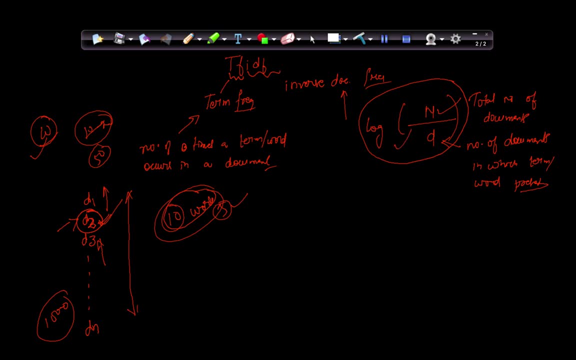 so this is, this is the intuition behind using this particular thing and how. this is how this is mimicking this intuition, how how we can uh formulate this intuition in mathematical formula. is this: n? n is the total number of document. okay, n is the total number of document and d is the. 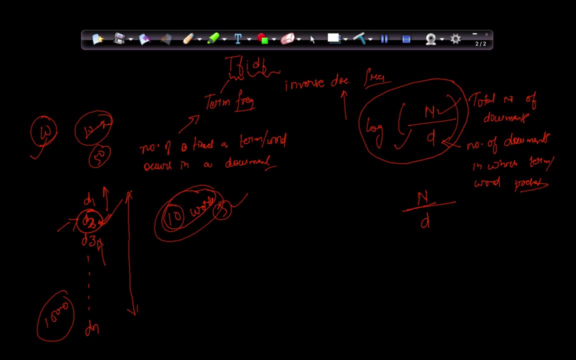 document in which the term was present. now, if suppose the number of documents is very large, suppose there are, uh, ten thousand documents- okay, there are ten thousand documents, and only in hundred documents that particular term was present, then the log of this particular value will be how much hundred? so log hundred. suppose the base is ten, then the idea value for that particular 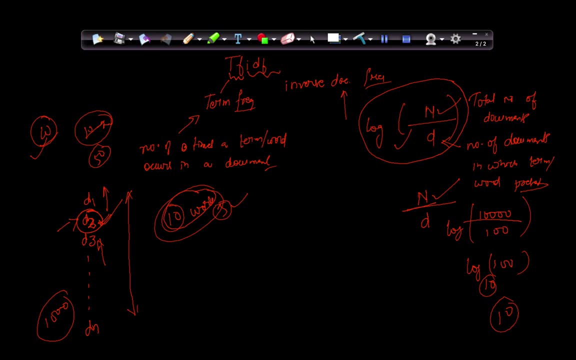 term for which we are calculating will be ten. now just compare. now, just for the comparison. for the first, suppose there is one another term or word w, for which, for which there are total ten thousand words, and that particular word, that particular word was present, in suppose two thousand documents. okay, so now cancel this one, and this is five. 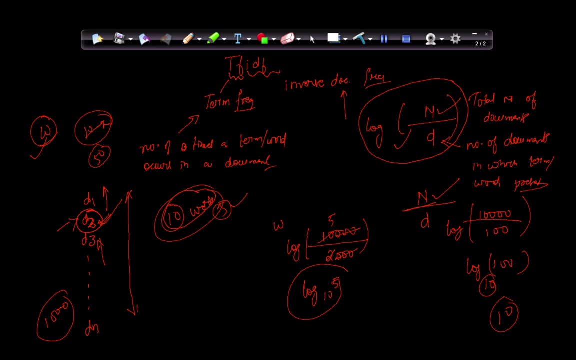 and log five: base ten. this will be a. this will be lot, lot smaller than this particular value, because this is ten and this will be less than one. so now, just for the comparison purpose, you can see that the words which are occurring rarely in our corpus by using this particular formulation, this this particular formulation. 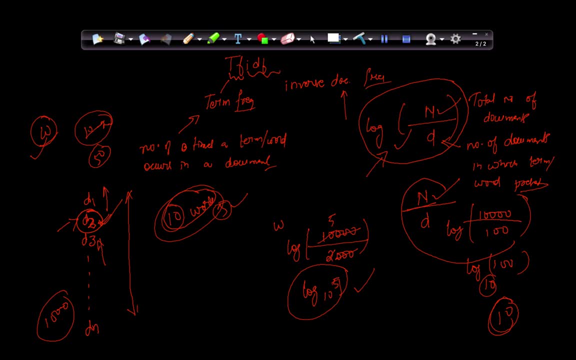 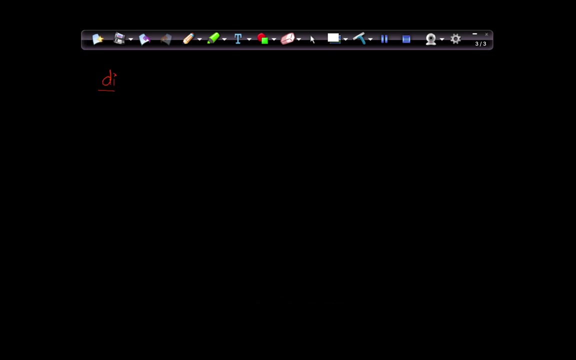 we can give more weightage to those terms or words which are very rare in our corpus. so now we will see what happens. now we have seen the idea thing, now we have to see the tf term and how we can get this. so now, now, suppose this is a document d1. it contains, suppose two: 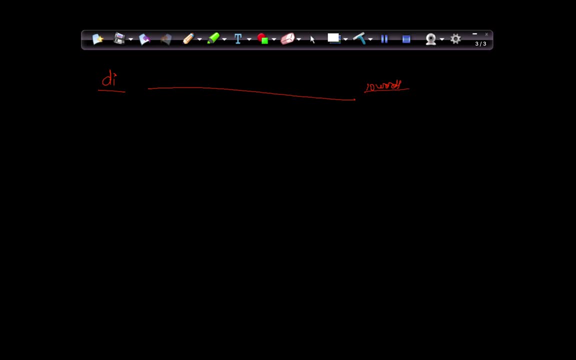 thousand words in total and we have an idea value of ten words, 10 words. so for every word we will have idea value because, because we have gone through the whole of the corpus, we have gone through the through whole of the corpus, now we have idea term. now this particular di is test. 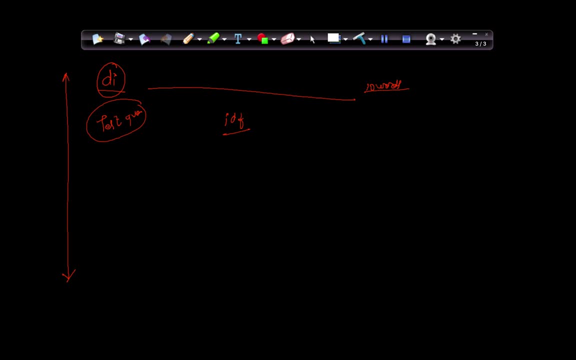 this is test query or this is at run time. suppose at run time a user gave a query: this is di and it contains 10 words. now suppose our vocabulary contains 10 000 words in total and we have idea value of ten words, values for every particular word. now what we will do is, while vectorizing, we will have 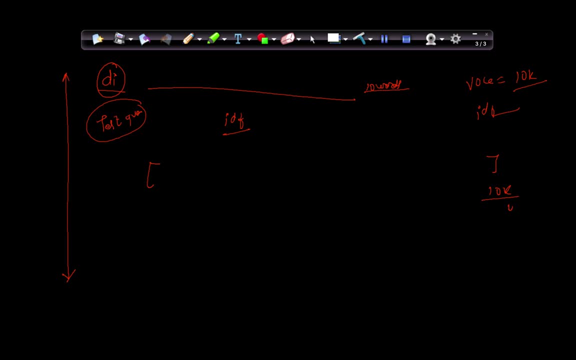 an array of 10k words, and at those particular indexes we will place tf, idf value. now what we will do is suppose this di contains 10 unique words and suppose each word has occurred two times, or suppose each word has occurred more than one times. so the tfi, the, the tf value for 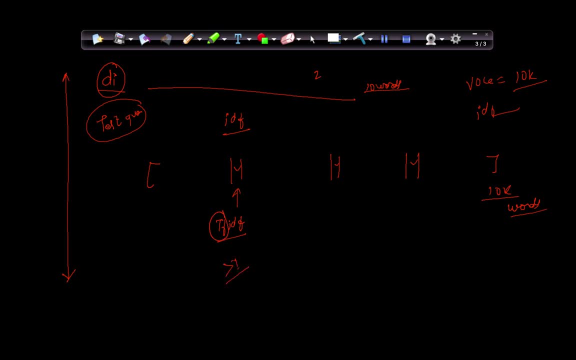 every word will be greater than one now because they have occurred more than once, and we will multiply the tf value with the idf value that we already have while we were fitting our tfi, the tf idf vectorizer. i will show you how to fit our tf idf vectorizer and get the idf values for. 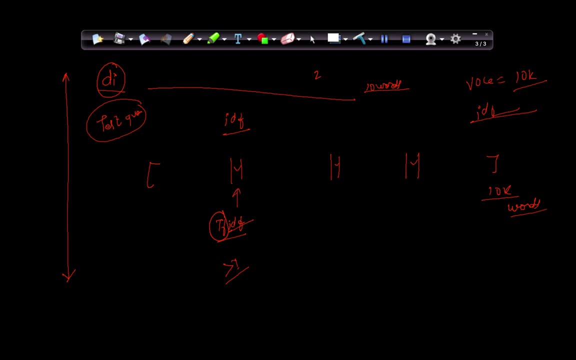 every word or the every unique word that we have in our corpus. now the words, suppose. suppose if this doc, this document, contain a word that is wn, which is not present in this particular vocabulary, then what we will do is we will just ignore this word, we will not. 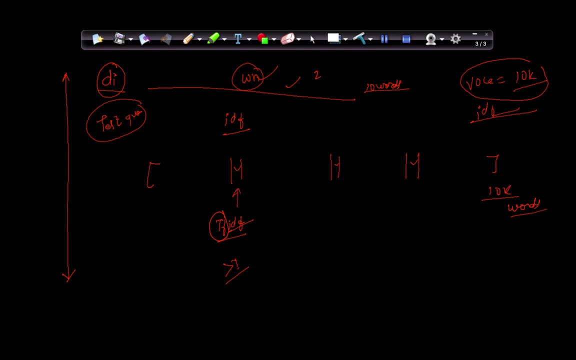 consider this word during vectorize and we will just behave in a way that this word was not present in our document. so the words that are present in the document, we will only consider those words, because once our vocabulary has been built, we cannot vectorize those words that are. 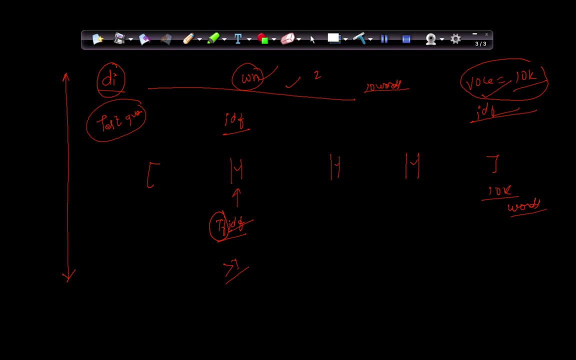 not present in this vocabulary. so once that has been done, we will simply calculate the term frequency. we have seen how to calculate it in our bag of words. we have idea values for every words. we will just multiply it and we will get it now in reality. for the 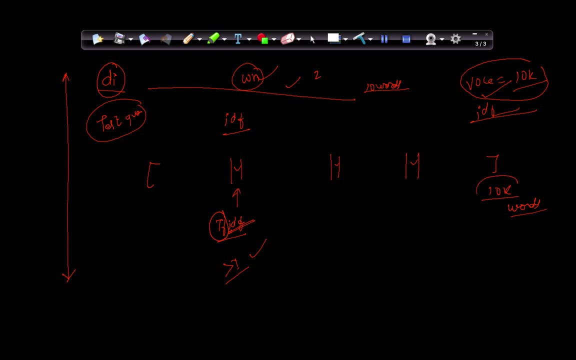 demonstration purpose. this is good, that we are having a, an error of ten thousand, an error of ten thousand just because our vocabulary size is ten thousand. but in reality we don't have this. what we do is we simply have the index number, suppose. suppose we have a word w1 and w1 has 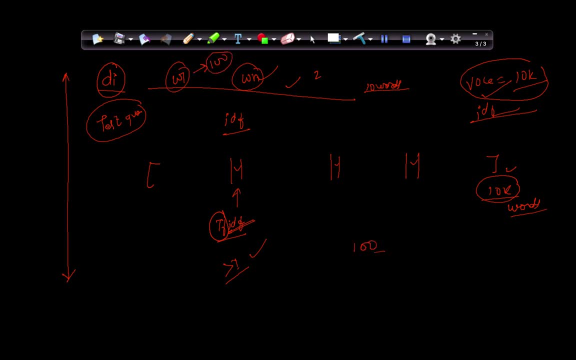 been assigned an index of hundred. so what we will have is we will have a of 100 and we will have the TF IDF value of this particular index. now suppose we have a word w2 and its index was 105. so we will have what we store is we will. 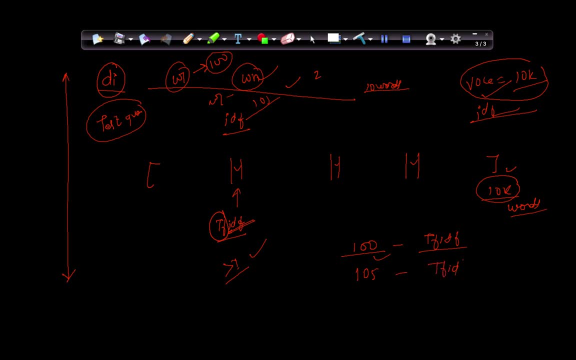 store 105 and we will store the TF IDF value of this particular word, because now word are represented by the index that was assigned to that particular word. now suppose we have a word w3 and its index is 201, so we will store 201 and we will store the TF IDF value of this particular word. so in this, 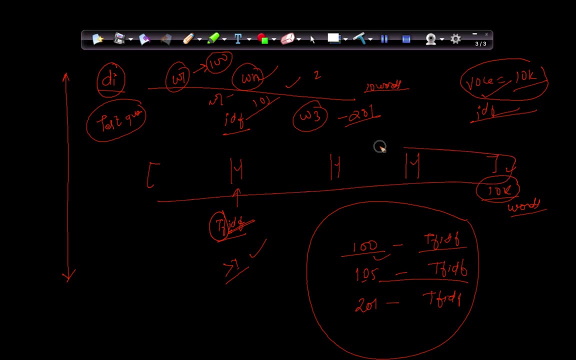 particular fashion we store. we don't have an array of this 10,000 words, and I will show you. so now let's move on to Jupyter notebook, and there we will see how to use TF IDF vectorizer. that is provided by the SQL and library. okay, now 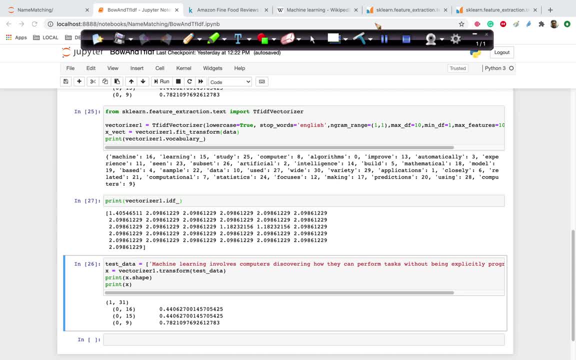 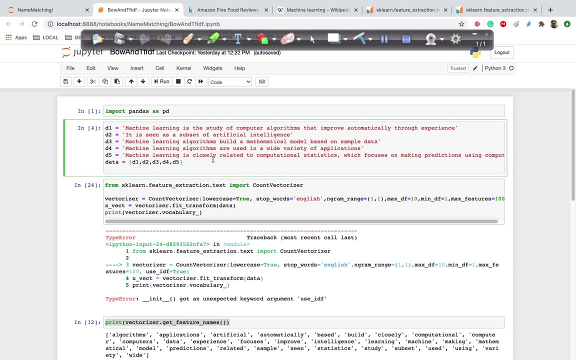 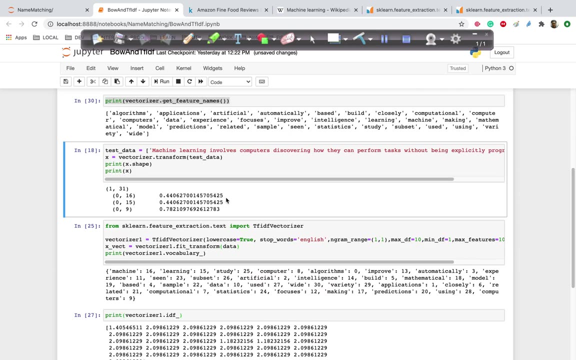 just move here. we will use the same data here also that we have been using till now, the same data we have seen here. this particular data now in. in my previous bag of words, video I- I forgot to show you how the vectorizer will vectorize the test data, so now just see here. suppose this is the query. this is the. 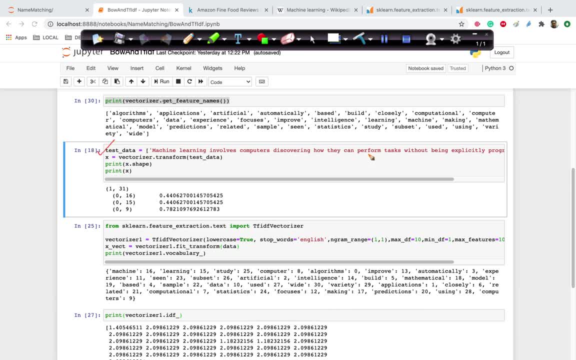 query that we have got from the user, this particular document, and now we have to vectorize it. what we will do is we will simply put this query in a list, we will pass the list to the vectorizer, and here we will not use fit transform, because fit transform should be called only once by 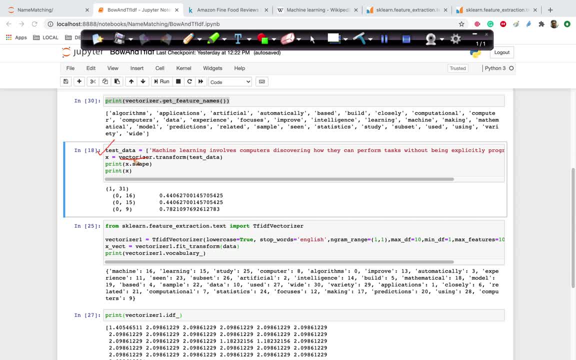 training once the vectorizer had been has been fit. we only, we will only use transform, because we just have to transform this particular query. we don't have to fit the vectorizer. we have done this when we were training. now, once the vectorizer is fit, we will transform the test data and now see, we have to print. 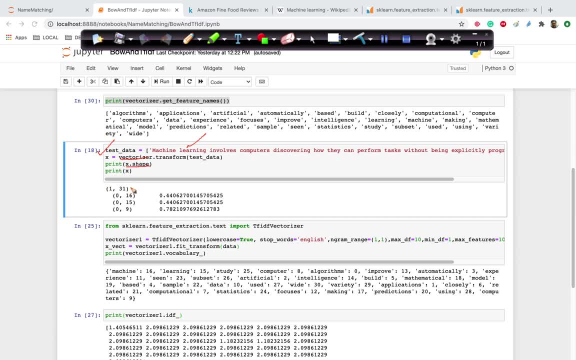 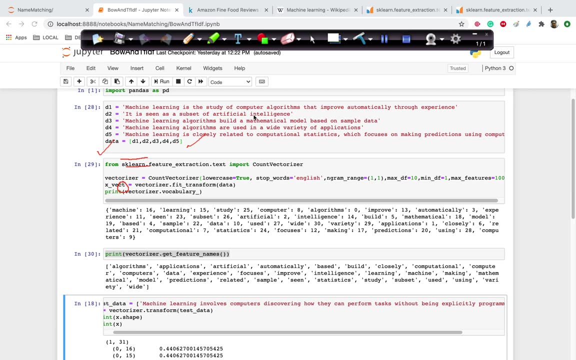 the shape X dot shape will print the number of rows and columns. this, this particular 31, indicates that we have 31 unique words in our whole of the training corpus. see, this is our training corpus. now, this is this is our training corpus. this is our training copper. this is very small, just for the 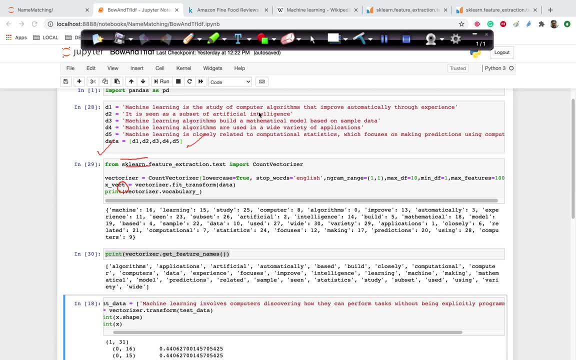 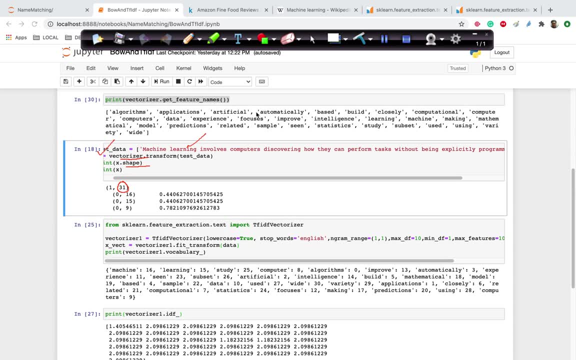 example purpose. in real life, we will have a very large turning corpus and where we will have millions of awards. so now, now, let's see here: we have only 31 unique words here now. now, when we will print this X, we have three values. this is 0, comma, 16. this is 0, 15 and 0- 9. what is this? 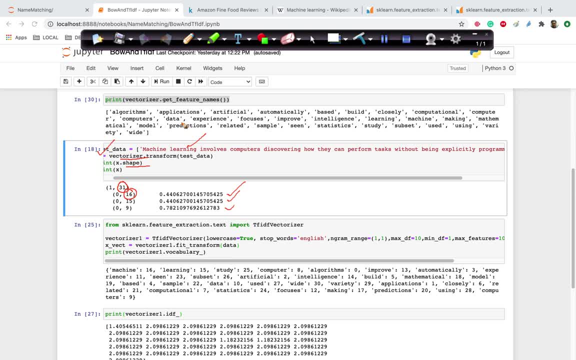 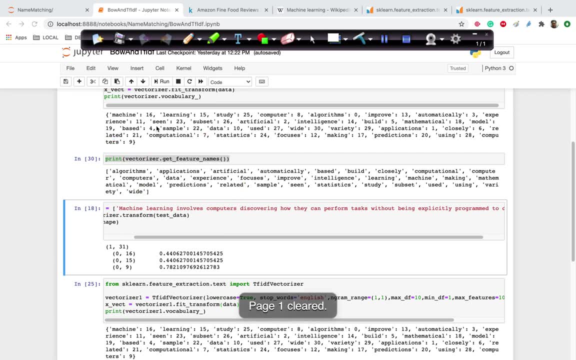 this is 0, 15 and 0- 9. what is this? this 16 and 0, 19. this is one. this is one is the index of the word. which word we can see here, which word this is, which was. which is the word that has an index of 16 you can just see here. see 16 was. 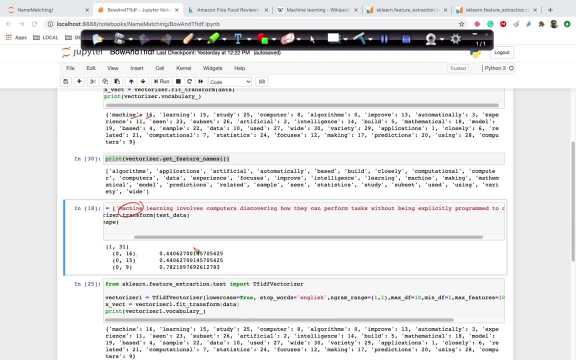 assigned to machine. so this machine was assigned 16 and the value that it has, that it has, is 16. now this one. now you can see 15. what is 15? 15 assigned to learning. so learning has been assigned this one and this is 9. what is 9? you can? 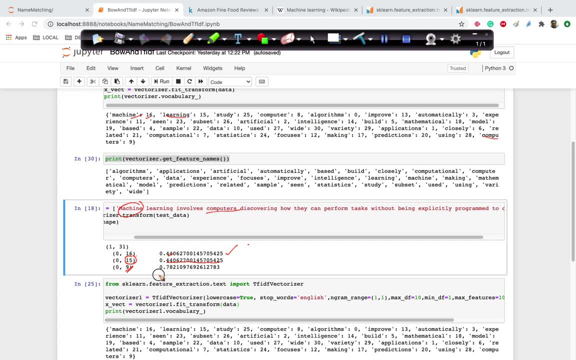 see 9. 9 is computers, so computers was assigned a value of this one. now rest of the values involves discovering how they can- so these are stop words- perform task without. so these words were not present in our vocabulary, so these words have been ignored. so I just wanted to show you how they are ignored and this value. 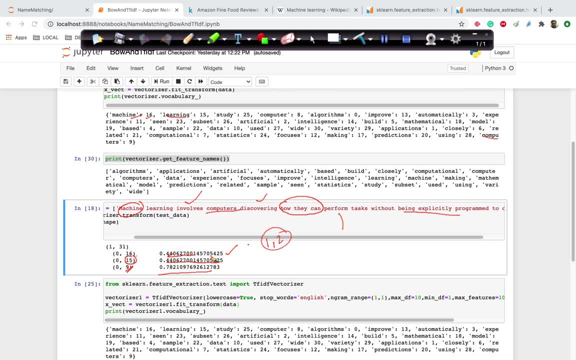 is not one, two, just because they have been normalized. so I will show you why we are normalizing this in our next videos, in my next videos. so now, now we will move on to tf-idf. now we will move on to tf-idf. so in tf-idf also, what we 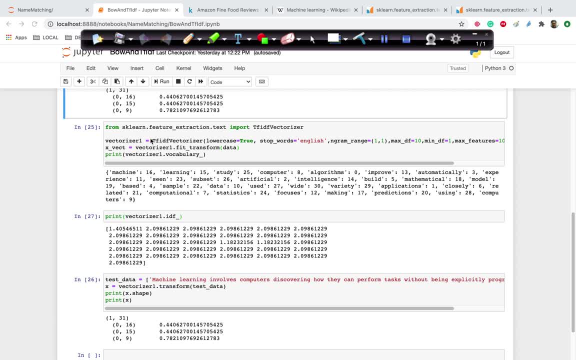 have to do is we will just first import the tf-idf class, we will instantiate that tf-idf class by passing those parameters. lower case: I have shown you stop words. I have shown you earlier n-grams. I have shown you earlier max df. I have shown you earlier minimum df. also, I have shown you. 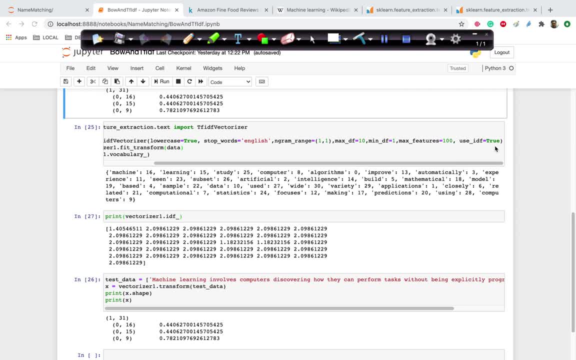 you max feature. source for now, use IDF equals to true. why I am using this one is this one is used. so if you want to see the idea values for every word in your vocabulary, I have just used this one to show you the idea values. now we 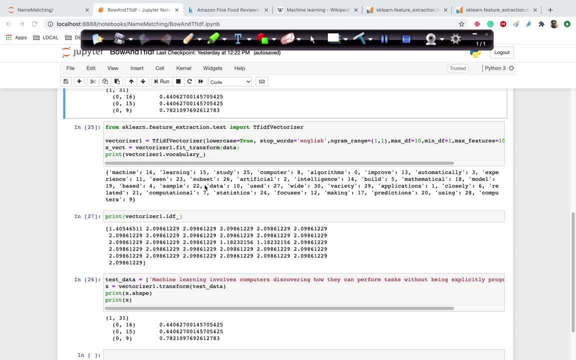 simply have to fit transform, we have to pass that data. you can see the vocabulary that was built. now, if you want to see the idea values, you just have to call this particular idea attribute. now this machine has this idea value, this learning has this idea value. this means their study has to point this value, to go in this way, so every 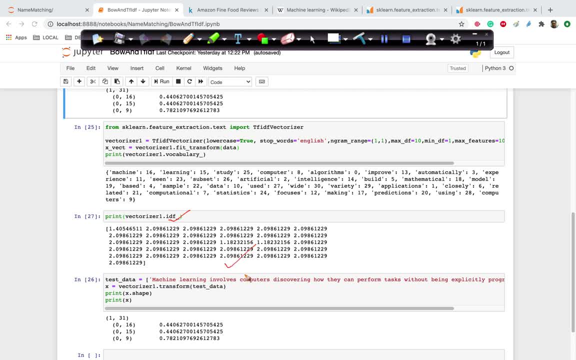 word has been assigned an idea value. yes, so you can see this. you can play around with this. I will share this notebook, along with this video also in the description link. I will share this Jupyter notebook now, while test data has been passed by the user. when we will transform this, these are the values that 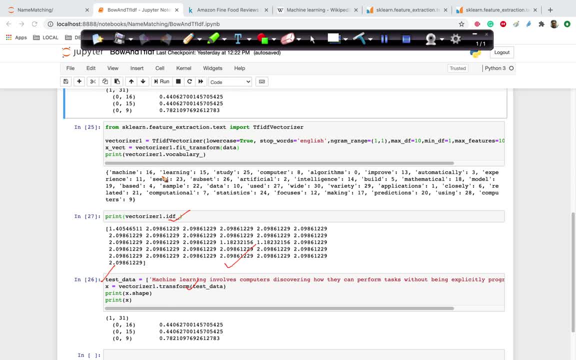 we are getting. why we are getting these values? because our training purpose is so small that the that bag of words and TF, IDF has don't have much difference in vectorization because there are very less words. once we will have a large corpus, then these values will differ a lot. so I think I have made my points. 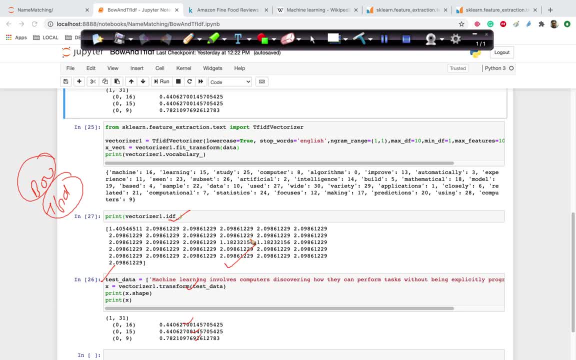 very clear and don't worry if you are not understanding it very properly. we will see all those things when we will do a real-life case study. when we use logistic regression to solve a problem there, we will use bag of words and TF, IDF, and you can see the difference in the performance of the models. when we 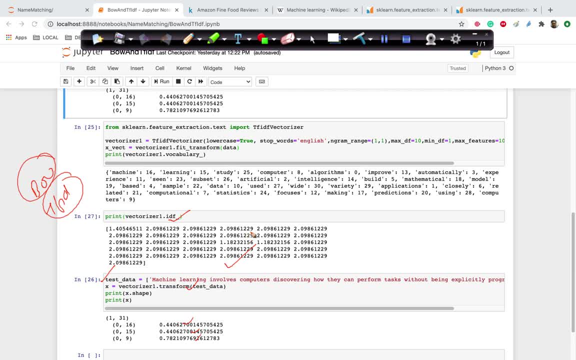 will use bag of words and when we will use TF, IDF, so you can see that. so if you are liking the video or if you are getting what I am making or the videos that I am making, then please consider subscribing to the channel, because I will be uploading videos on every topic each week, and each week at least I will. 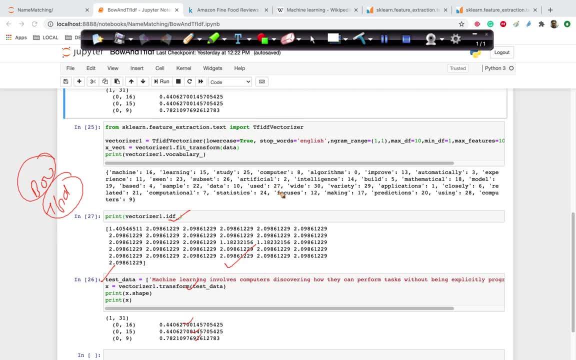 upload 10 to 12 videos so that you can cover machine learning very fast, you? so that's for now and thanks for watching this video. 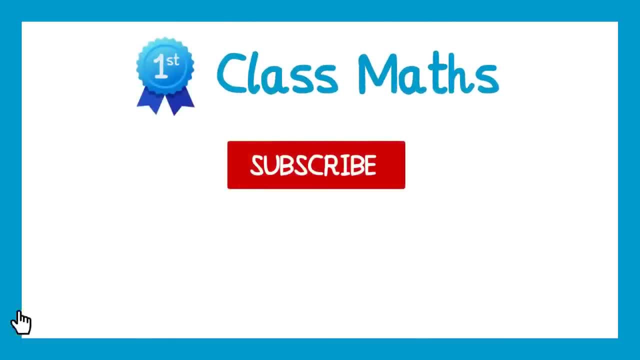 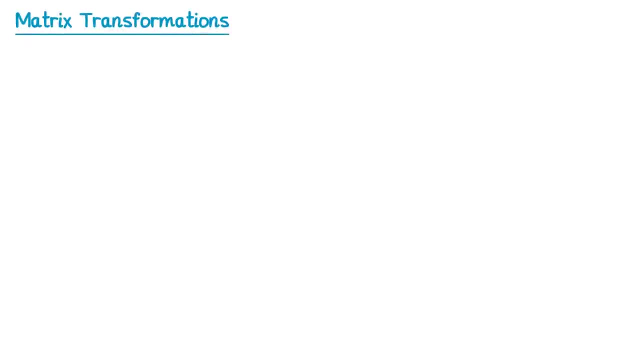 In this video we're going to learn how to do matrix transformations. You'll find some exam questions in the video's description that you can try afterwards. We previously learnt how to multiply matrices. For example, if we take a 2x2 matrix and a 2x1 matrix, we can multiply them. 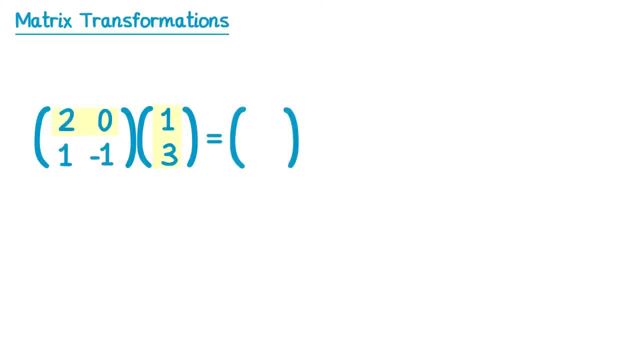 We do 2, 0 and 1, 3. So 2 times 1 is 2 and 0 times 3 is 0, and 2 add 0 is just 2.. And then we do 1 negative 1 with 1, 3.. 1 times 1 is 1 and negative, 1 times 3 is negative 3. So 1 take 3 is negative 2.. 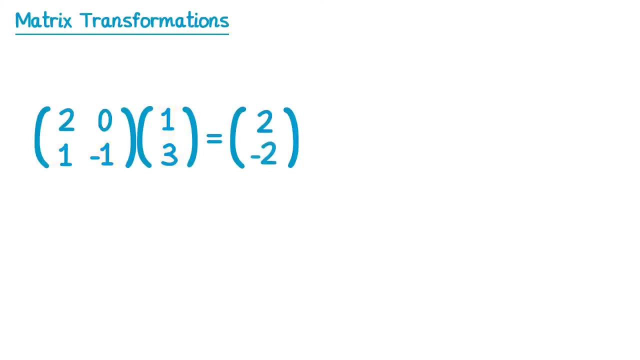 Now, when we're looking at matrix transformations, we want to imagine that each of these 2x1 matrices actually represents a coordinate. So if we look at the matrix 1,- 3, imagine the top number, the 1,, is an x coordinate and the bottom number, the 3,, is a y coordinate, Then we've got the coordinate. 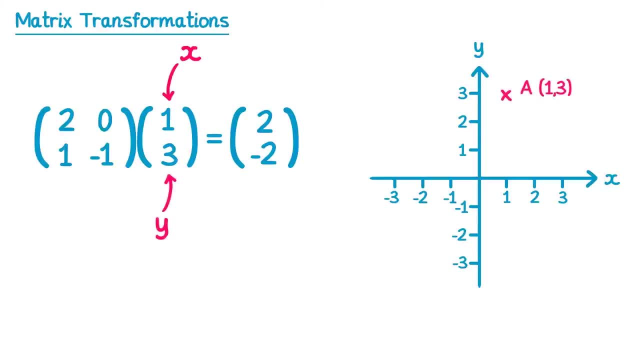 1, 3.. Let's mark that and call it a. Now let's look at the other 2x1 matrix, which was the result of the two matrices together: 2, negative 2.. Again, the top number will be x and the bottom number 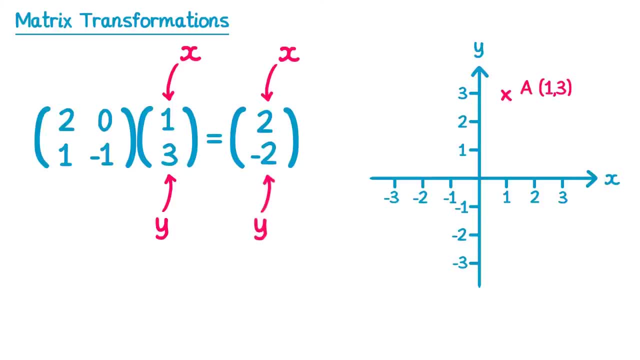 will be y. So we've got the coordinate 2, negative 2.. We'll label that a dash. So what we've shown here is that if you take a point 1, 3 and then multiply it by that matrix- 2, 0,, 1,-